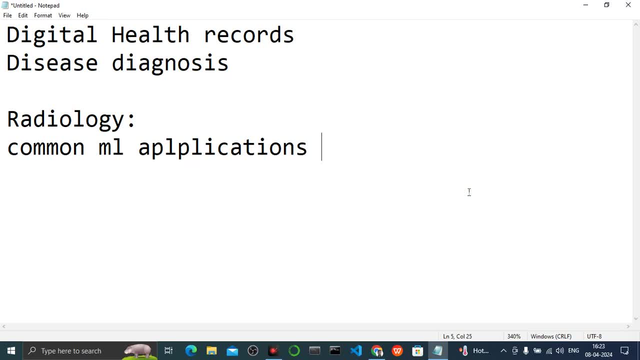 Hey folks, so we'll get dive into the video particularly So let's get understand about now Let's get dive into the working with healthcare data set. We will be looking at very small Python code implementation with healthcare data set. This will enable you. 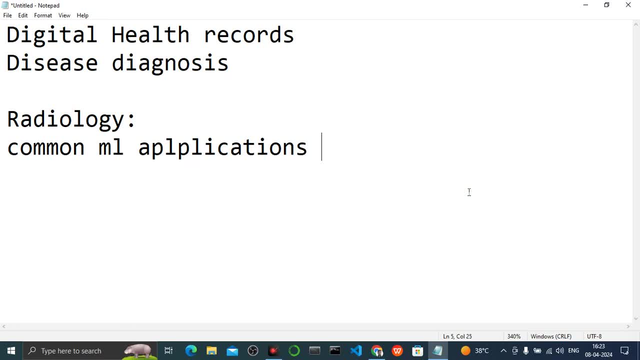 to understand how machine learning is applied in healthcare domain. in practical terms, We are using the Python 3.x version to run this code, So procedures to install some Python libraries is given. We will be going to do it, So you will be going to understand. 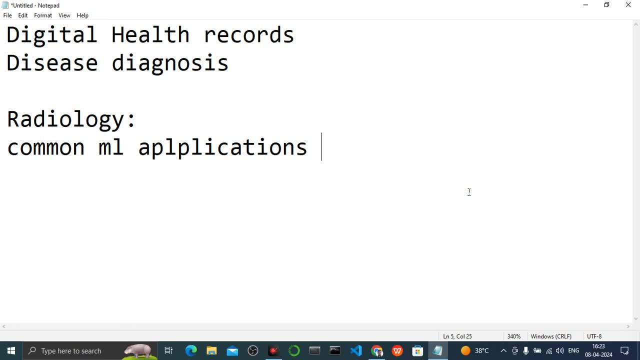 and I will be going to guide you. what are the things? we have to do it? Before we start to look into the machine learning and applying the prediction models to the various data sets, I would like to bring a disclaimer to you that none of the data is being used in. 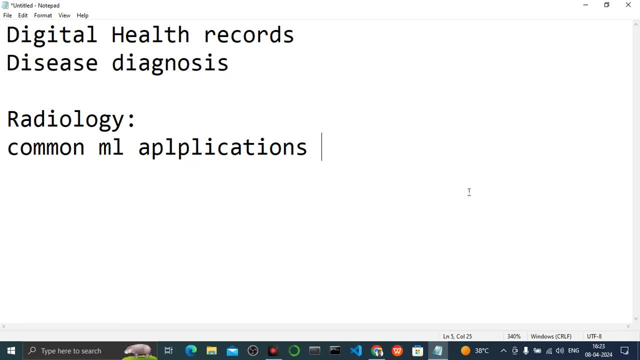 the exercise, It's belong to one of my clients or anything? Okay, it is a real patient in real world. Any resemblance to any data set that word is merely a coincidence, So neither the, neither me nor any things takes in responsibility for authenticity of a privacy. 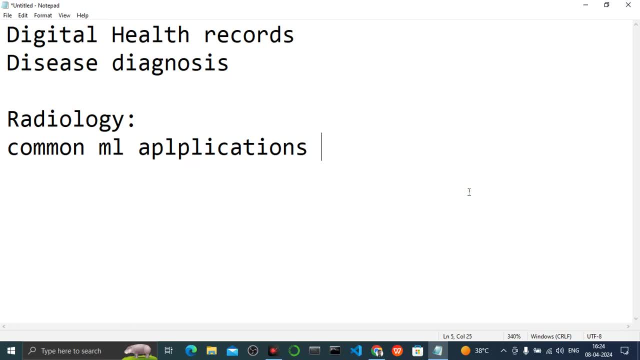 of this data set? Okay. so purpose or purpose of medical data set is to able to understand, like, how you can apply machine learning in healthcare data set in the production environment. Okay, the data set cannot be used for any other purpose, Okay, such as clinical trials or any. 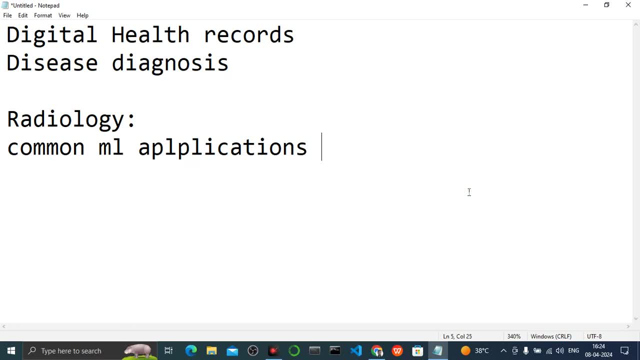 production or commercial related activities. Okay, electronic or otherwise. Okay, so let's get dive into the video. Now I will be going to explain the life cycle of the machine learning development, basically. So in the market, you will be going to tell us, like data science, life cycle. 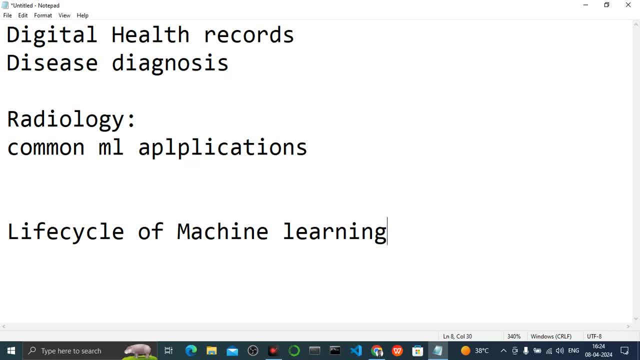 data science life cycle, machine learning, life cycle. what are? what are the things that are going to be used for any other purpose? Okay, so just clinical trials, or any production or commercial. what are the things that are going to be used for any other purpose? Okay, machine learning. 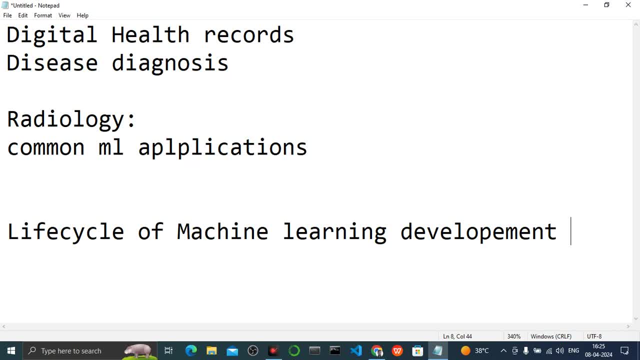 development. in certain books they will be calling it as machine learning development, data science life cycle. Okay, so that is a main key difference here. So, before proceeding to the look at the data set, like building the machine learning models, let's, let's, let's to the let's. 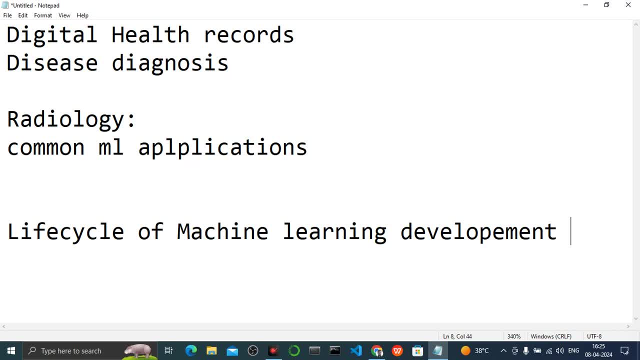 look at like what are typically machine learning life cycle and it is and is and learn its implementation within a short application. This is a general life cycle model that I will be going to explain how this can be applied to any machine learning application development. So it's not a just a healthcare, but also you can apply to into any domain. 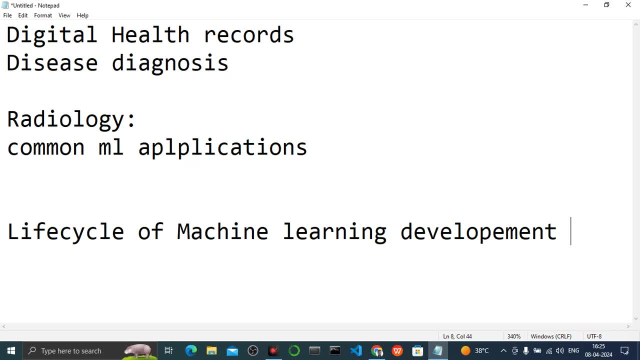 any domain like retail finance sector, like that may be a transport or anything, logistics or anything, Following step by step approach. that person carries out the machine learning in their application. does not get lost in any important parts of the process. are able to complete the machine learning application as as as a professional standards. 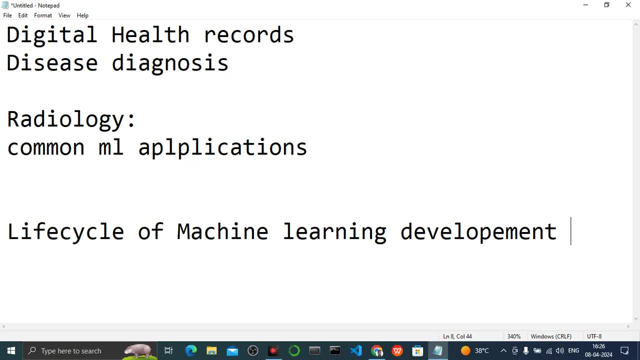 basically, Though this model does not have reference, any reference because it's based on the experiential, like my experience, knowledge with the years of working into the machine learning application for my clients and I'm giving you giving- to the lifecycle process. basically Alright, so let's get dive into the video and we'll just try to. 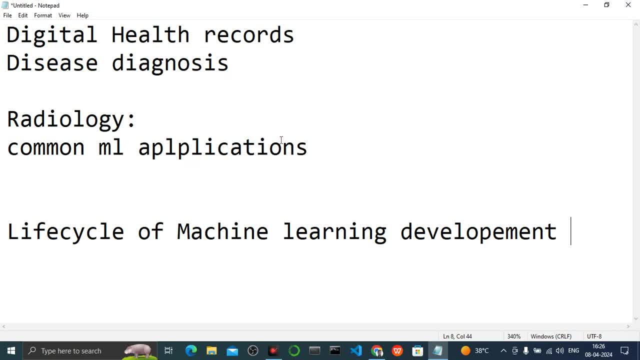 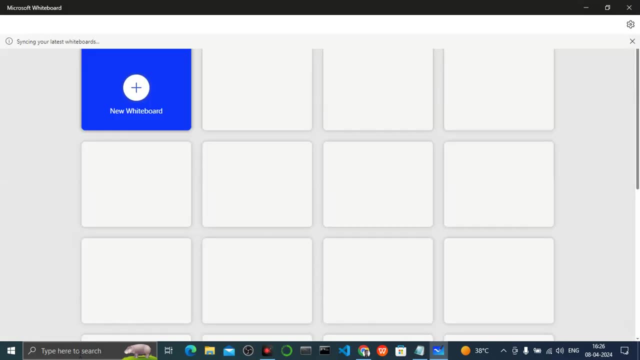 write one particular lifecycle so that you will understand very clearly. So I will be going to take it as a whiteboard So you will get to understand what each and every steps it is going to tell And we'll be going to understand that part. Okay, Alright, we'll just take the another. 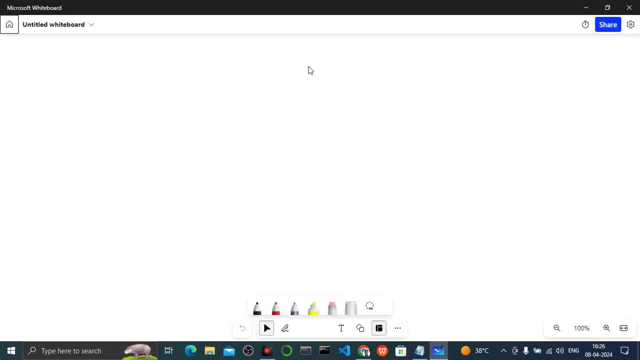 whiteboard So that you will understand What what I'm going to talk about. Alright, so we're just going to take this, use this template. Okay, so I will be going to take this, Okay, So in the between, this is a machine learning. 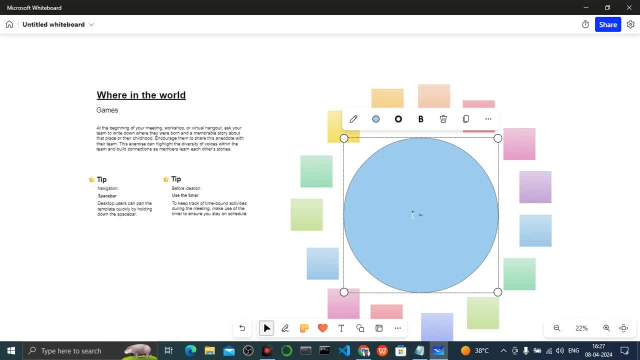 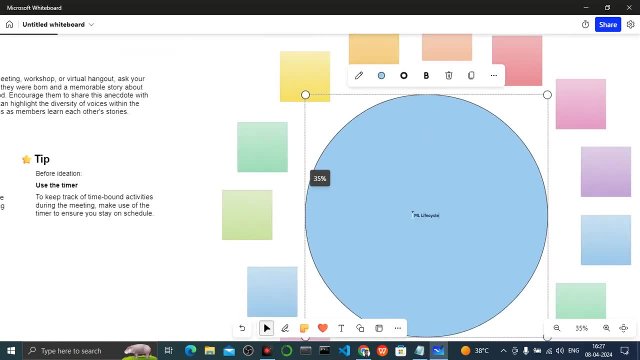 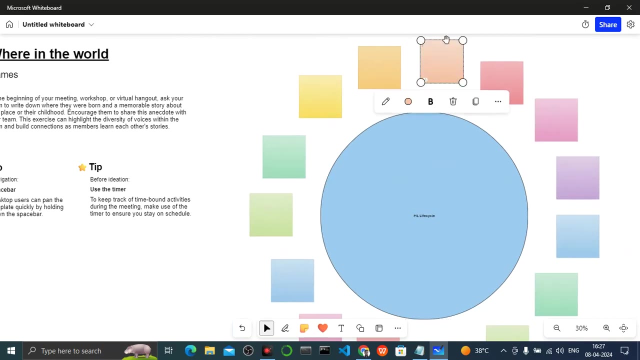 lifecycle, Okay, And then lifecycle, Okay. So if we just, if you just see here it is a life cycle, Okay, Okay. So what I'm going to take is here, here it is Business need, basically business need, business need, Okay, Alright. after the business need just: 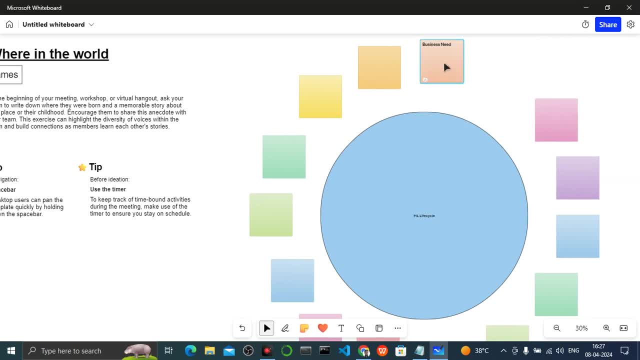 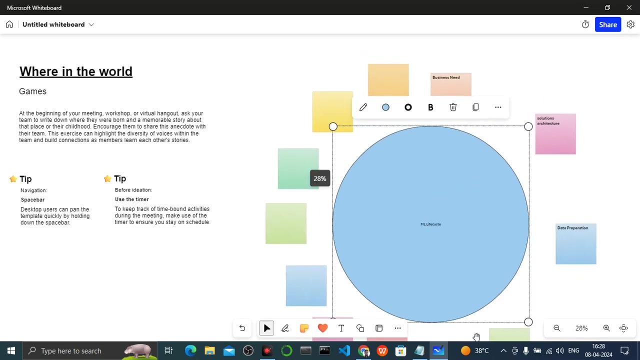 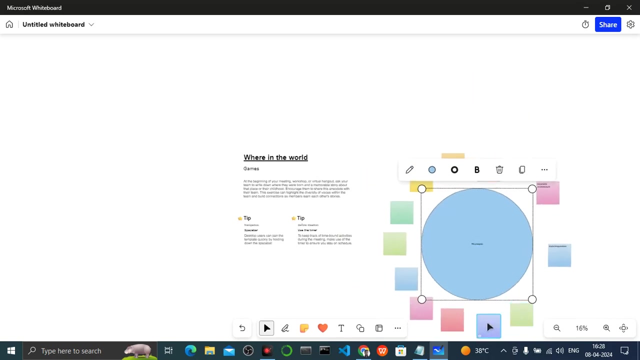 you move this, which is not required. Business need: alright, Business need then solution architecture. What will the architecture of solution? solution architecture: Okay, then data. Then comes the data preparation, data preparation, then data preparation, then EDA model building. 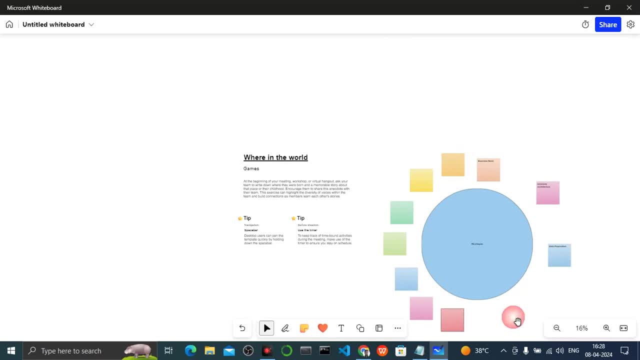 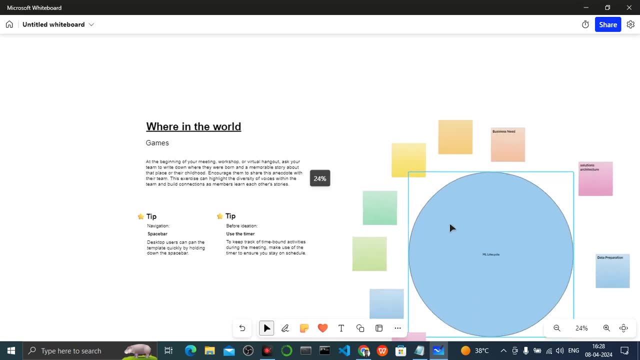 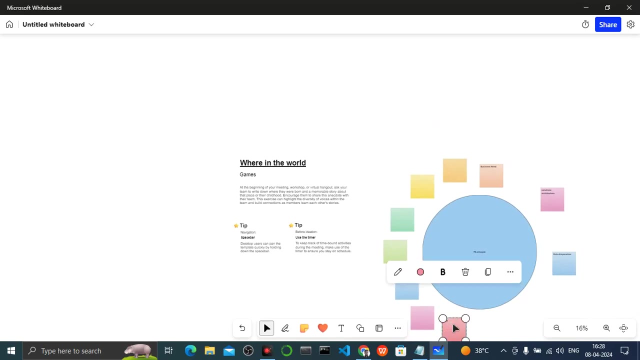 okay, all right, so we'll just stream it these things. so this is a EDA. EDA is nothing but exploratory, exploratory data analysis books. okay, so don't. uh, let me just stream this. okay, so it is a EDA. EDA, model building, model building. 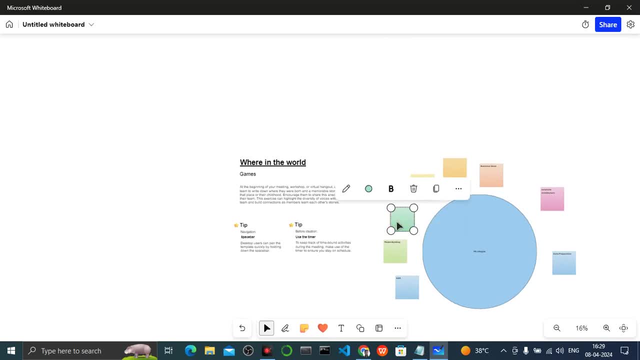 model validation, model validation, modern validation. then it comes the model implementation and feedback: model implementation implementation and and feedback and feedback. all right, right, so then we will be considering to the business needs itself. okay, so this is, this is a life cycle of this. basically, okay, so we'll just try to make. 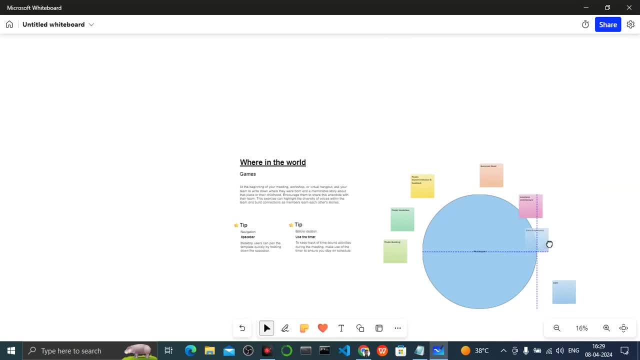 it very more structured, okay, all right, we'll make it like this. we'll make it like this. you can make it like this. okay, it will be made more structure, right? so this is the things, folks. okay, so these are the life cycle which you wanted to do it. so what's each or each stages will do? we're going to talk about it, okay, so. 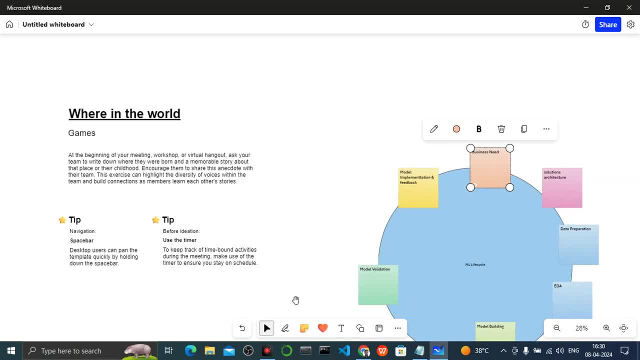 we'll just try to understand, okay. first is a business name, and what you can do is here. you can just write it like this, okay, so we'll just write it like this. just just copy this, okay. okay, so we just paste it like this, basically. so it. 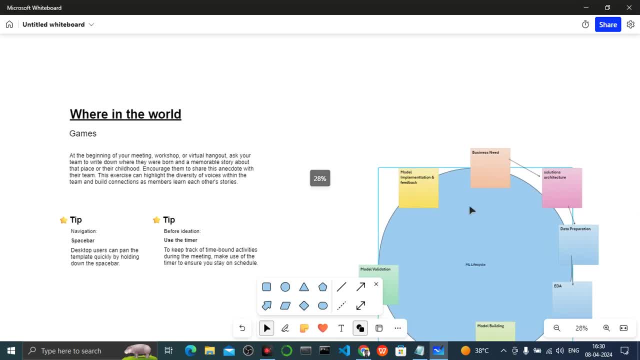 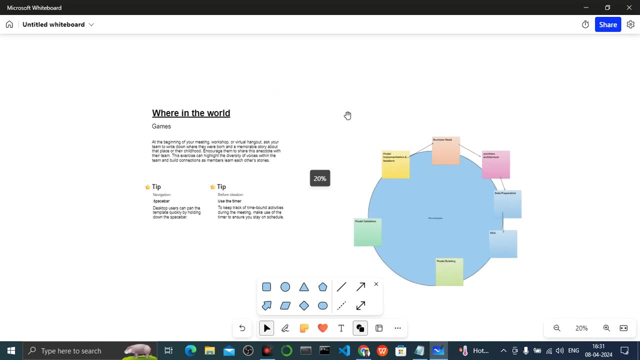 will be very easy, right. so then it will be like this, basically: model implementation feedback. once again: you do here, okay, so you do like this, so like this, okay, all right, so you can just do like this, basically okay. so what we do is we'll just take this, just paste it, okay, so this: 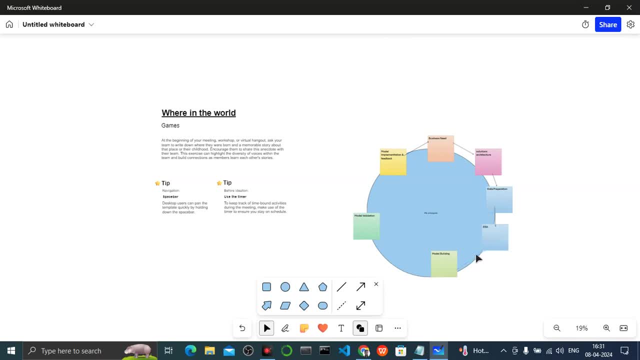 will be like this, then it comes okay. so it will come okay. so this is a like one way, basically okay. so life cycle: basically it is a machine learning life cycle in yourself. framework, basically all right. so business is to key to any machine learning application is provides a justification. 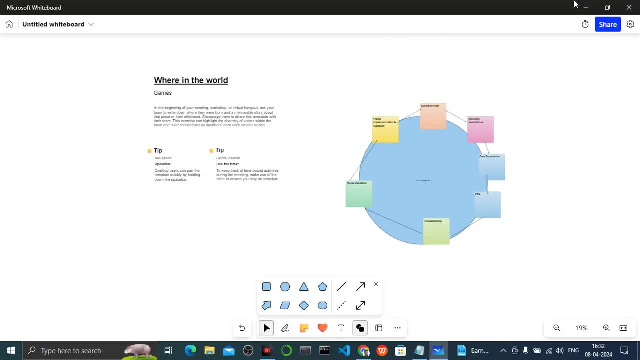 for need resource during the life cycle development. business need is like something. we can go different various stages of life cycle so that team implementation for the object does not lose the sight of the original goal. okay, so next step is to creating machine learning solution architecture. during this process, we will process it with the machine learning engineer and data science team. 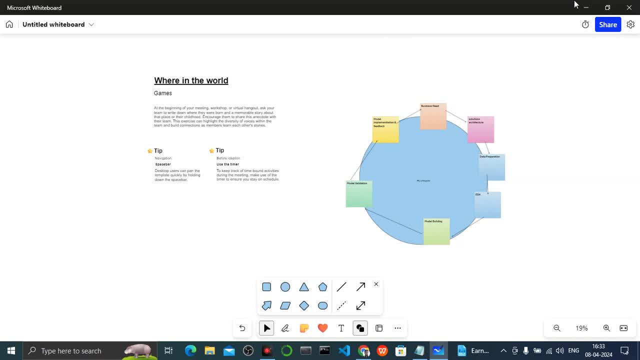 that is a set out of, to create a template based out of which machine learning application would be created. it is during the stage: conceptualization of the business, translation of the business, leading to technical architecture, tech space. it is also part of a life cycle, okay, where the 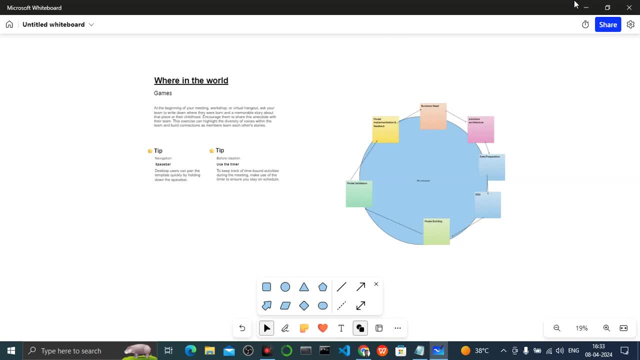 architects of the machine learning application go back to the business in order to understand they need better to start translating into the machine learning application the implementation solution. so next stage will be the data preparation, where it is very important phase because right from the data we need to identify what kind of a data is required for. 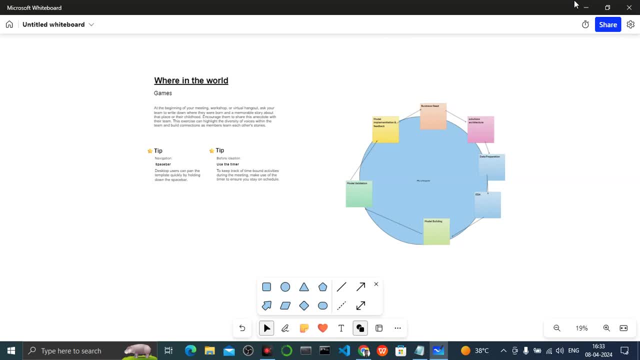 identifying the sources from where it will come. once we know the data is required for the organization where the application is being built and it needs from the outside of the team that is being building from. the machine learning solution requires it with whole data set is big. okay, then it at least sample data set can be used. it will build the most of the tasks. 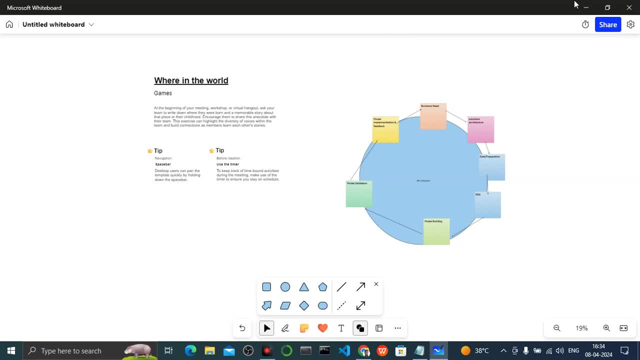 determine what kind of format the data is available. okay, classification is made like data is available in such a spread fast, like dot, csv, xml, json or oracle database or db2 database, etc. okay, so classification is made by the implementation team, regardless. what is the source of structured data? what is the source of unstructured data? treatment of unstructured. 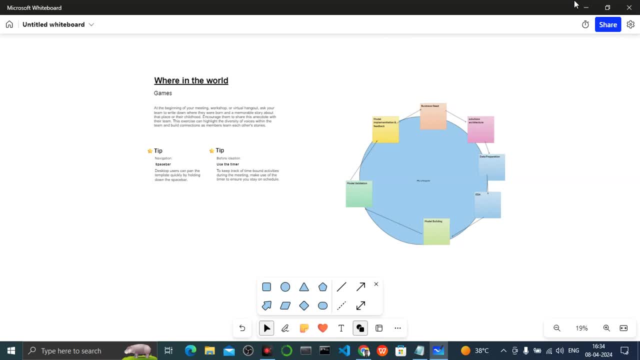 data, structured data in a machine learning are very different, hence data wrangling, which we largely deals with. the cleaning of the data, okay here. all such data does not add any value to our business solution. so need is elimination and only that data is required for solving the business. 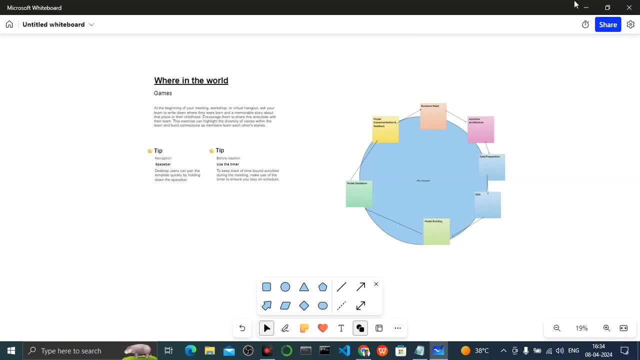 need is kept once the data cleaning happens. next, the step of machine learning life cycle, which is eda. in eda we look the basic statistics of the data, such as mean median score and its correlation between the different labels. we need to identify whether the data is comprised of numerical or categorical variable, etc. 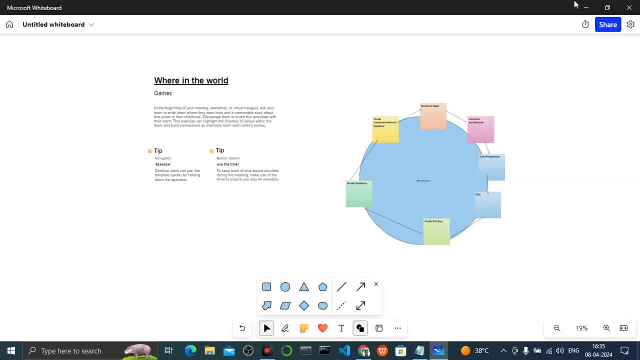 okay, so when the eda gives the direction to the model building, for example, the choice of algorithm will depend on different kind of variables that we have. okay, so now in this sample, we may have a data sets with categorical variables, such as gender maker- male or female- to be predicted based on the other labels. in such case we may have to use 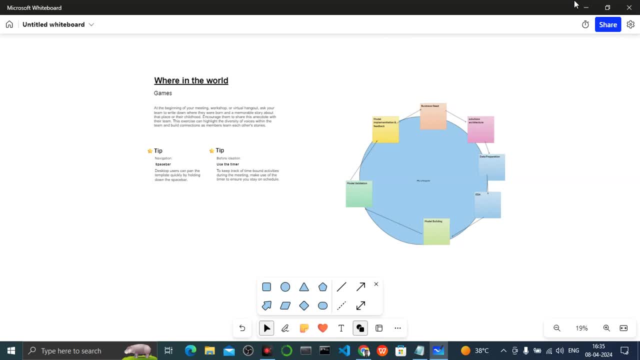 non-quantitative algorithm for our model building. model building is a next step and is closely tied up with the eda. in the process we do analysis, descriptive statistics, we identify which model, we identify which modeling technique we are going to use. then we will build a benchmark predictive. 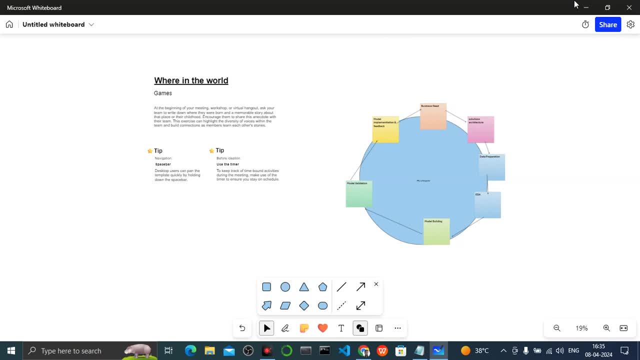 model. we use other models and algorithms on the data set and we try to interpret, find the best algorithm for creating the predictive model. once the identification of model is done, the next step is to create the model validation. we use the good results. then the model is deployed and it is. 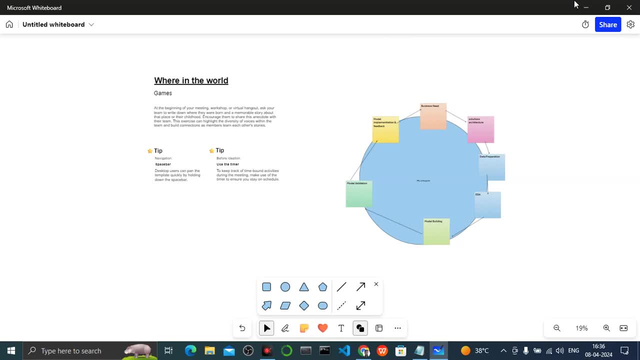 implemented okay. after the feedback is taken. we use the good results. then the model is deployed and it is implemented okay after the feedback is taken to see if it has met for the business need for which it has it was built. okay if there is a new business need or the model needs to take care of some things of the business. 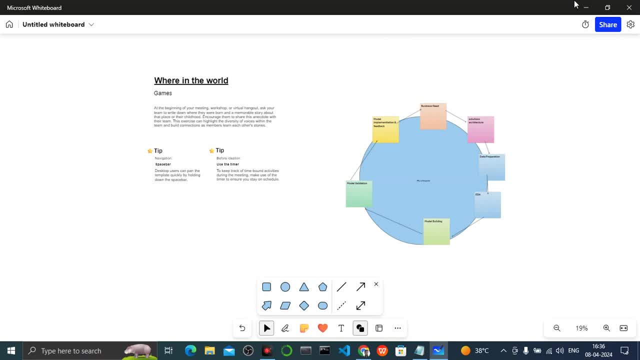 requires. then we again, we go back to the process of solution architecture, data preparation, media model model building and do the model validation, in essence, of the life cycle process. we that goes on. machine learning application is terminated. okay, so like this we will be going to do business: major solution architecture, data preparation, eda model building, model validation.